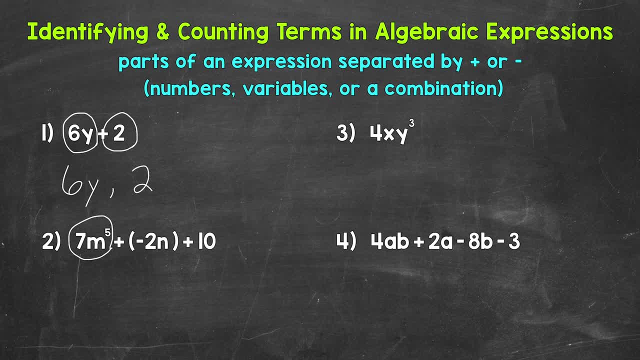 So we can see that this is the first part, the first term. So 7m to the power of 5.. Then we have plus Negative 2n, So this is the second term, negative 2n, And then we have an addition sign and then a 10.. 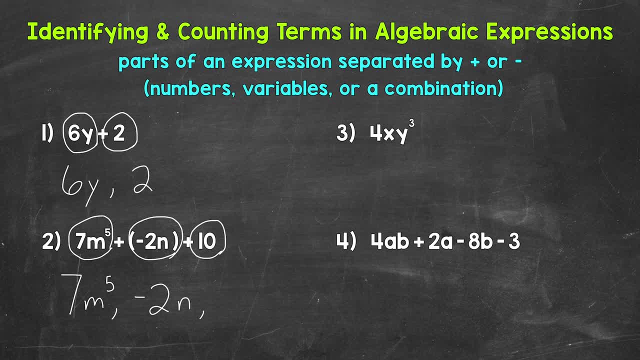 So we end with this 10 here, and it's a positive 10.. So for number two we have three terms: 7m to the power of 5, negative 2n and then 10.. 10., 10.. 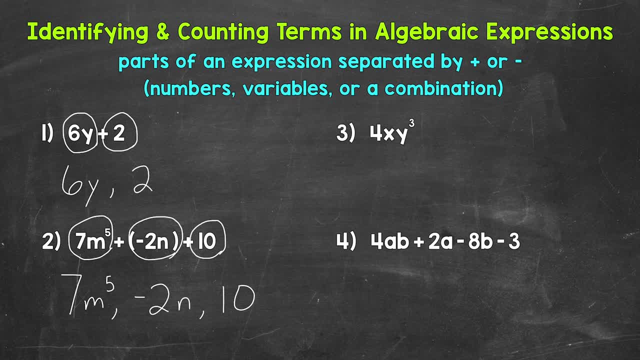 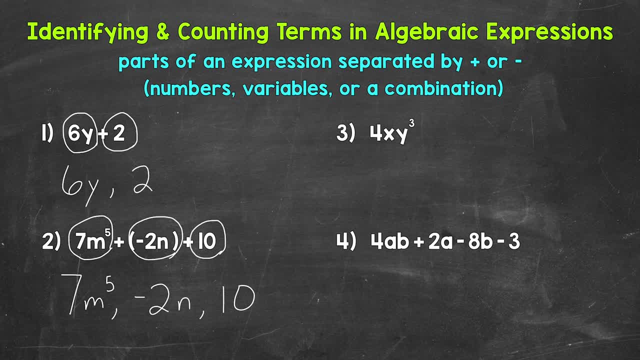 Let's move on to number three, where we have 4xy cubed. So for this algebraic expression we don't have any addition or subtraction signs. So this is actually one term. We only have one term here: 4xy cubed. 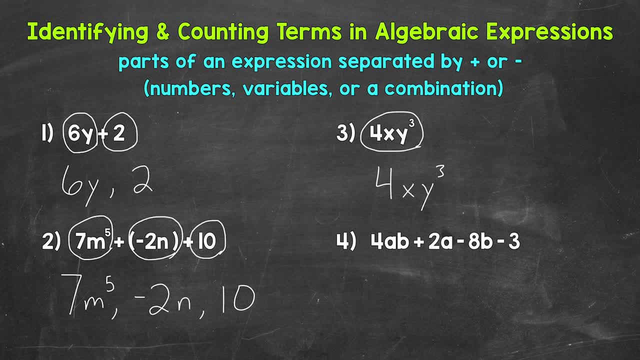 And that's okay. We can have algebraic expressions that are just one term. Lastly, let's move on to number four, where we have 4ab plus 2a minus 8b minus 3.. So let's look for the parts, the terms that make up this algebraic expression. 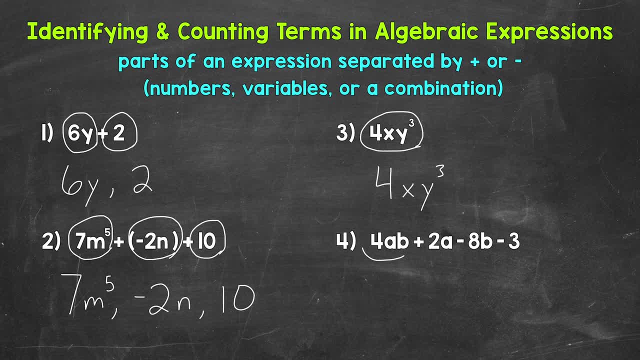 We'll start with 4ab, So we have 4ab, 4ab and then an addition sign, So we can see that this is our first term. Then we have that addition sign and then 2a, So 2a is the second term. 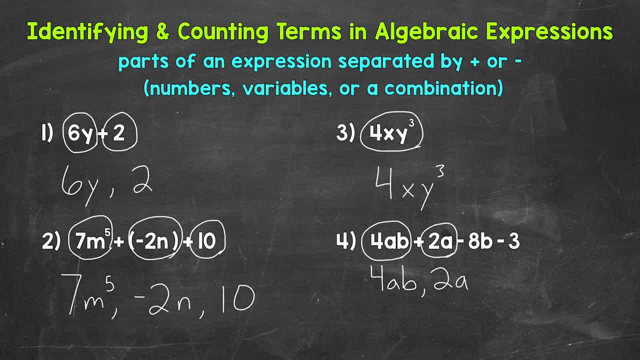 And it's a positive 2a. And then we have a subtraction sign that separates the 2a from the next term where we have 8b. So we are subtracting 8b, 8b. Again Terms take the sign that's in front of them. 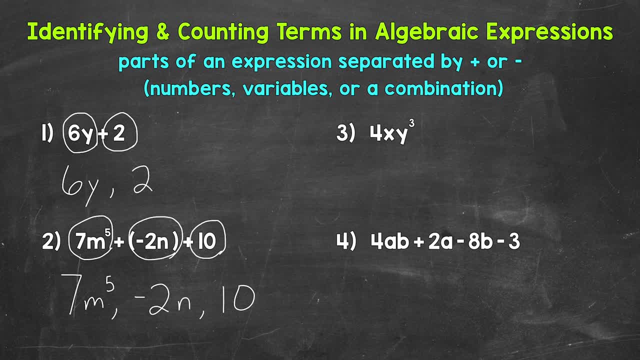 Those are the parts, the terms that make up that algebraic expression. Let's move on to number three, where we have 4xy cubed. So for this algebraic expression we don't have any addition or subtraction signs, So this is actually one term. 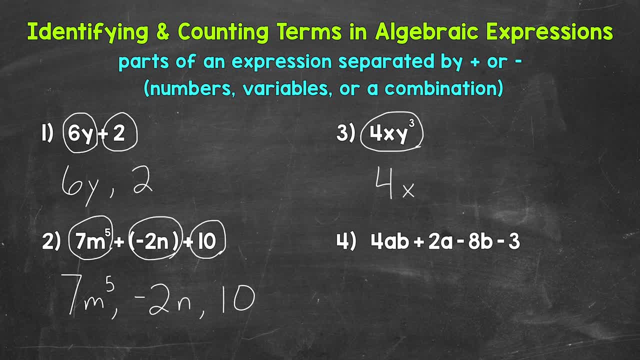 We only have one term here, 4xy, xy, cubed, and that's okay. we can have algebraic expressions that are just one term. lastly, let's move on to number four, where we have 4ab plus 2a minus 8b minus 3, so let's look for the parts, the 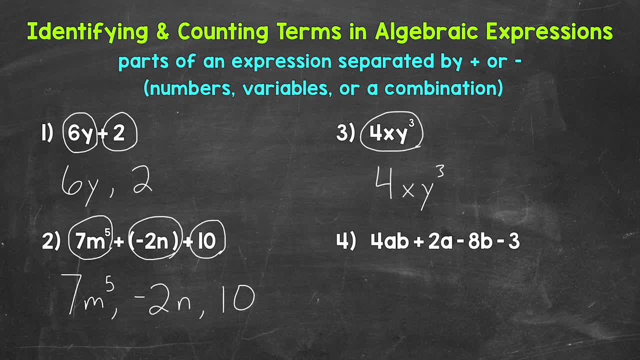 terms that make up this algebraic expression. we'll start with 4ab, so we have 4ab, and then an addition sign, so we can see that this is our first term. then we have that addition sign and then 2a, so 2a is the second term and it's a positive 2a. and then we have a subtraction sign. 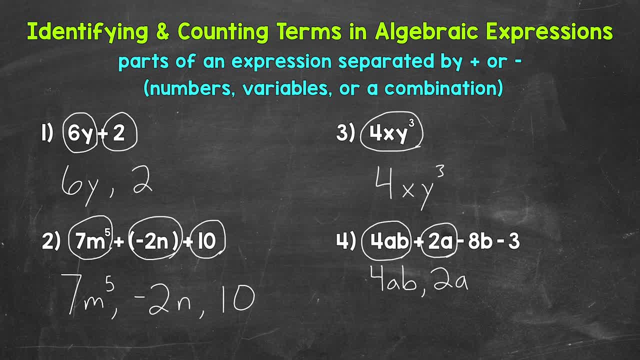 that separates the 2a from the next term where we have 8b. so we are subtracting 8b again, terms, take the sign that's in front of them, so this is a negative 8b. and then, lastly, we are subtracting 3- again, take the sign that's in front, so this is a negative. 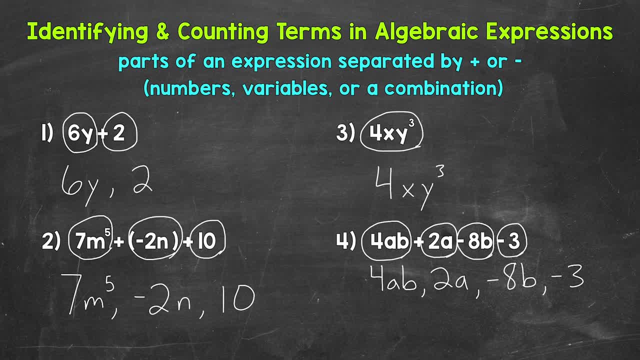 3. so for number 4 we have four terms: 4ab, 2a, negative 8b and negative 3. now, before we end here, i do want to mention one more thing, and it's about rewriting algebraic expressions using only addition. this will make it a little simpler to identify terms, especially the negative ones. 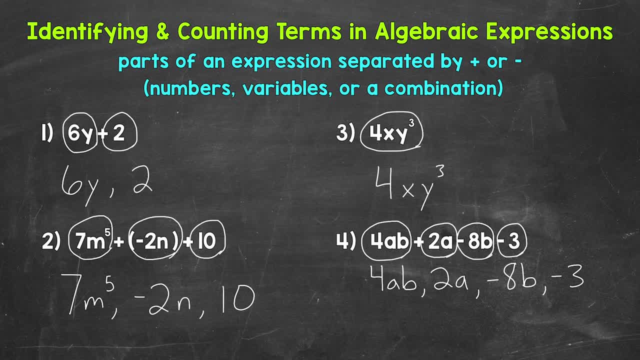 because everything will be separated only by addition. now we can rewrite algebraic expressions using only addition, by rewriting subtraction as adding the opposite. so, for example, where we subtract 8b sogar age, maybe that's a positive number, just to let you get a picture of what's. 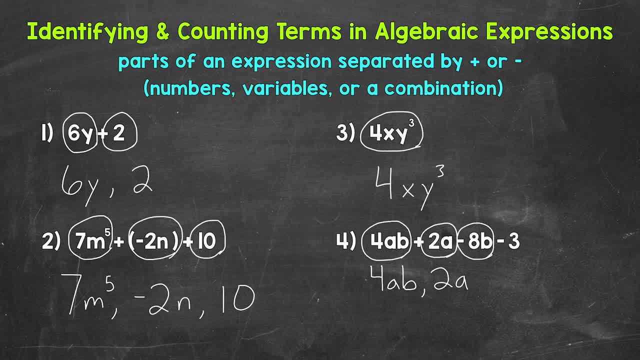 So this is a negative 8b. And then, lastly, we are subtracting 3. Again, take the sign that's in front, So this is a negative 3.. So for number four, we have four terms: 4ab, 2a, negative 8b and negative 3.. 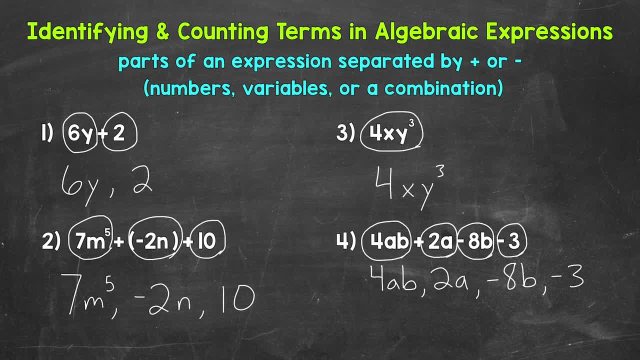 Now, before we end here, I do want to mention one more thing, And it's about rewriting algebraic expressions using only addition. This will make it a little simpler to identify terms, especially the negative ones, because everything will be separated only by addition. 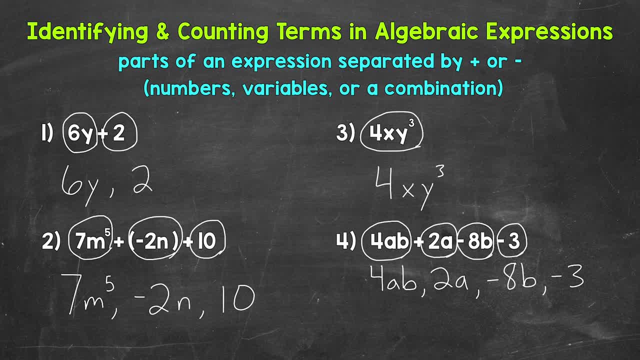 Now we can rewrite algebraic expressions using only addition by rewriting subtraction as adding the opposite. So, for example, where we subtract 8b, we need to add the opposite. We are subtracting a positive 8b, So let's add the opposite. 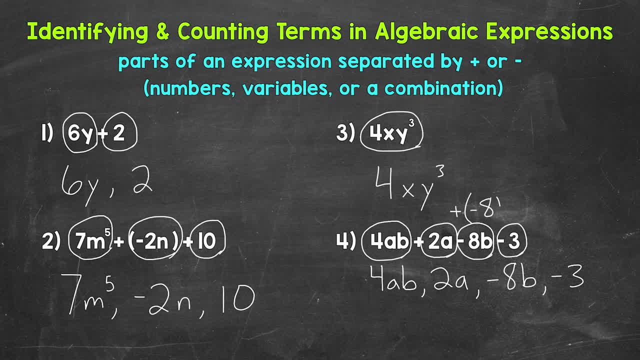 The opposite of a positive 8b is negative 8b. Then we are subtracting 3. So add the opposite there. We are subtracting a positive 3. So let's add the opposite, So adding a negative 3.. 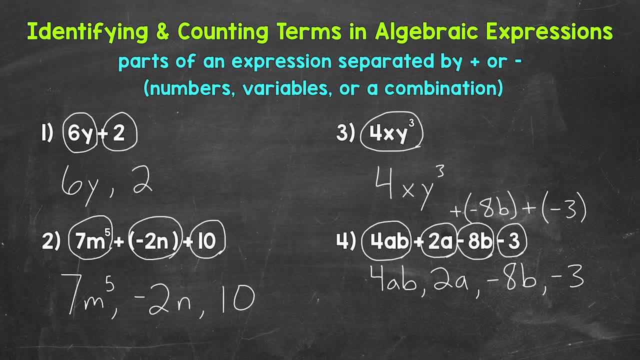 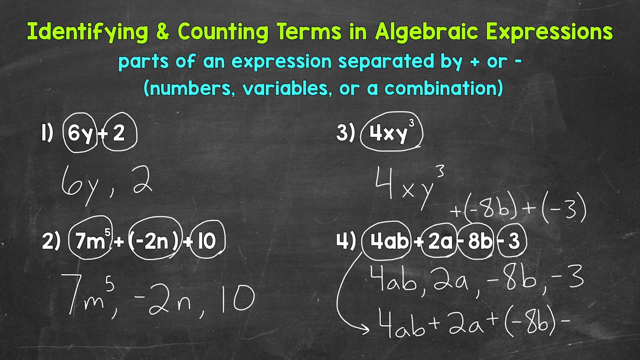 That's equivalent to subtracting 8b And then subtracting 3.. So let's rewrite that algebraic expression. I'll come below here. So we have 4ab plus 2a plus negative 8b plus negative 3.. 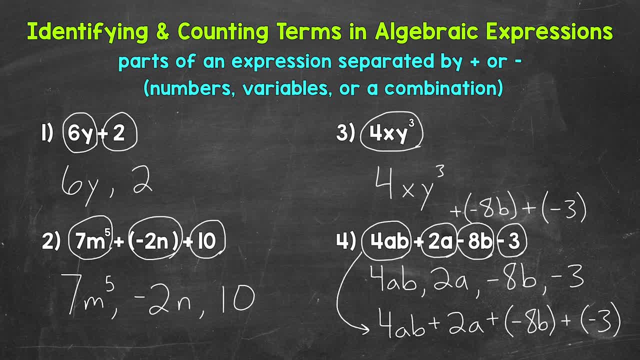 So those two expressions are equivalent. We're not changing the value of any of them. We're just changing everything to addition Again, by changing subtraction to adding the opposite, And you can see that we have the exact same terms: 4ab, 2a, negative 8b and negative 3.. 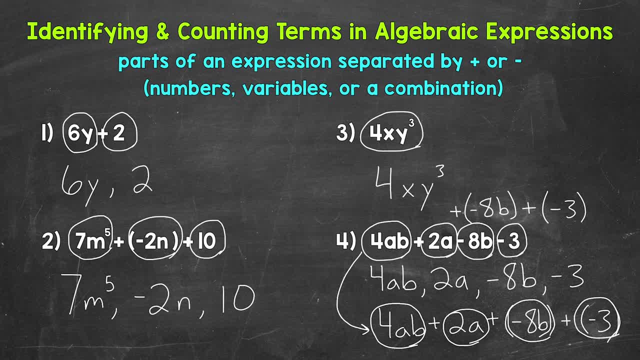 So it's a strategy to keep in mind. You don't have to do that, But again something to keep in mind. So there you have it. There's how to identify terms. There's how to identify and count terms in algebraic expressions.